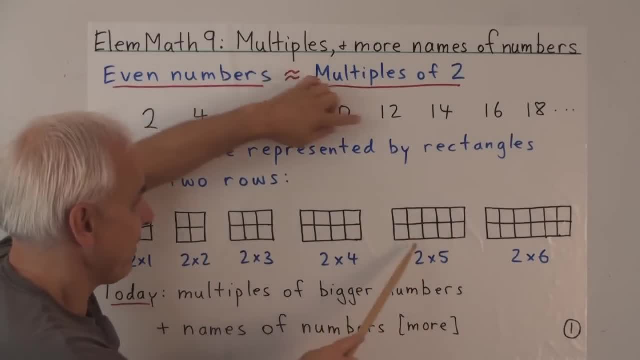 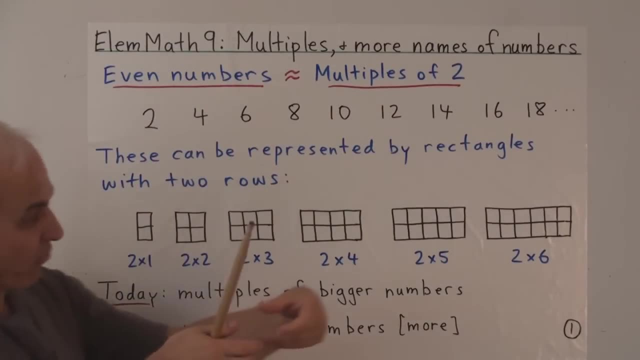 8 by a, 2 by 5.. 10 by a, 2 by 5.. 12 by a, 2 by 6. And so on. So all of the even numbers can be represented by rectangles that have exactly 2 rows. 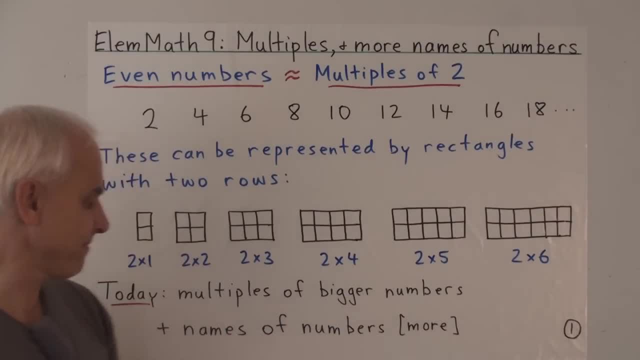 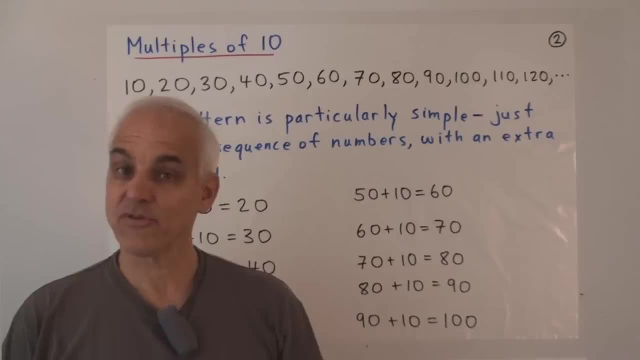 So today we're going to look at multiples of bigger numbers And we're going to talk then about the names of numbers a little bit more than we have already. So, after the multiples of 2,, probably the next simplest multiples are those of the number 10.. 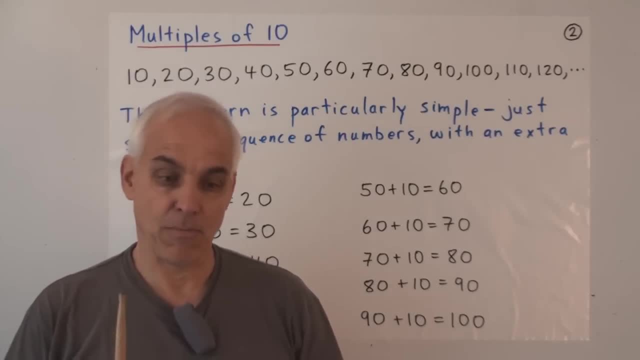 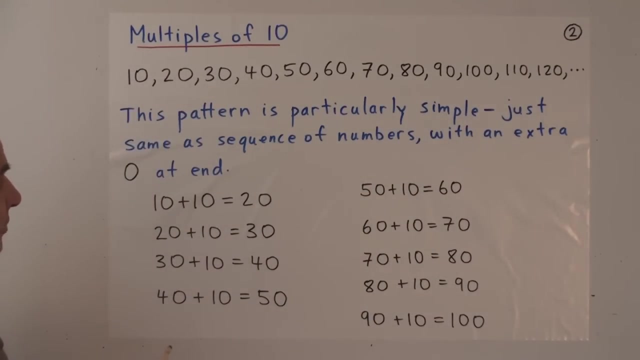 And that's only because we're working in base 10.. So multiples of 10 have a particularly simple representation and a particularly simple kind of arithmetic. So here is the pattern of multiples of 10.. It's a reasonably simple pattern because you see just the ordinary pattern of numbers. 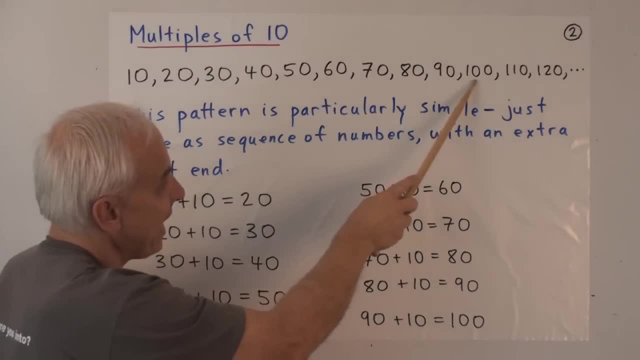 1,, 2,, 3,, 4,, 5,, 6,, 7,, 8,, 9,, 10,, 11, and so on, Repeated, Repeated, with an extra 0 at the end of everything. 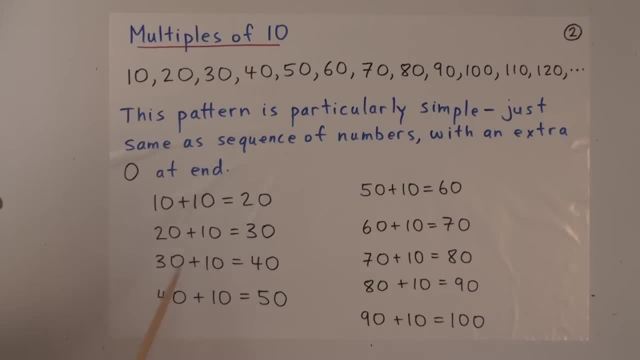 So how do we get this sequence? Well, the first one is 10. And then the next one is 10 plus 10. And that's 2 10s, or what we usually call 20.. Then if we add 10 to that, well then all together we have 3 10s. 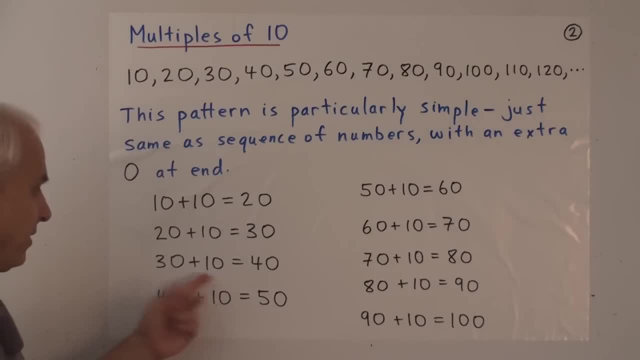 So it's represented by 3: 0.. We add another 10, and all together we have 4 10s, So it's 4: 0.. And so on: 5: 0,, 6 0,, 7 0,, 8 0,, 9 0.. 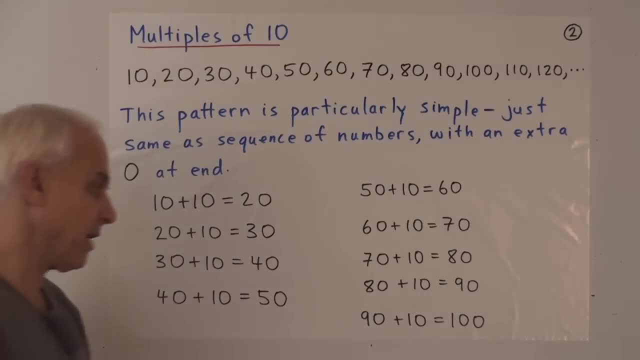 And then this number, 1 0 0, representing 0 1s, 1 10, and 1 100.. Because, remember, once we have 10, 10s, that's the same as what we're calling 100.. 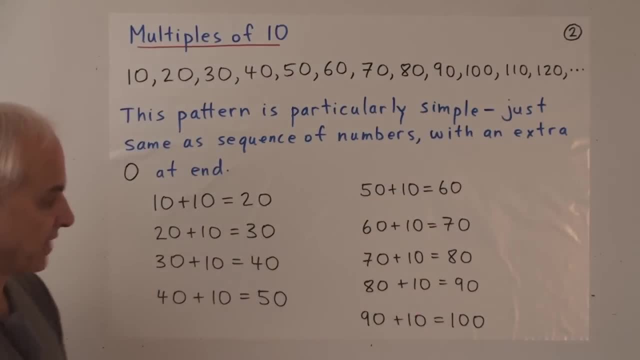 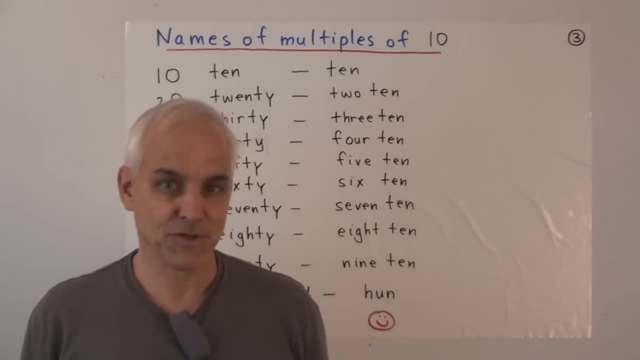 Okay, so we're going to be concentrating mostly on these multiples of 10, just from the range 10 to 100, at first. So our first order of business is to give some names to these multiples of 10.. Right now we have 7.. 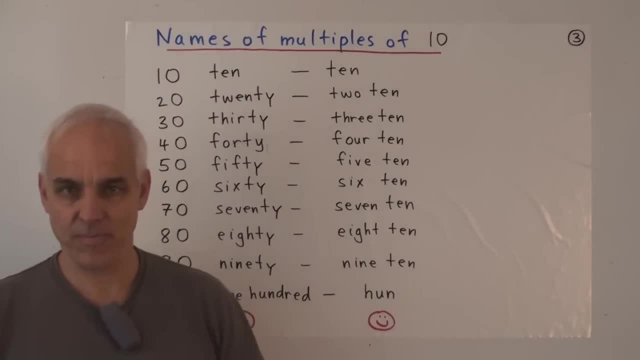 We have symbols for them, but we don't actually have names for them. So these numbers are important numbers and they get special names. Each one gets a special name, Just like the numbers from 11 to 19 or to 20 get a special name. 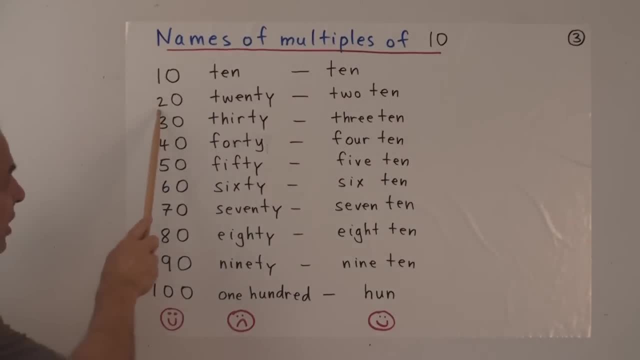 This one, we've already called it 10.. This one here we call 20.. The next one 30.. The next one 40.. The next one 50.. The next one 60., Then 70., Then 80., Then 90.. 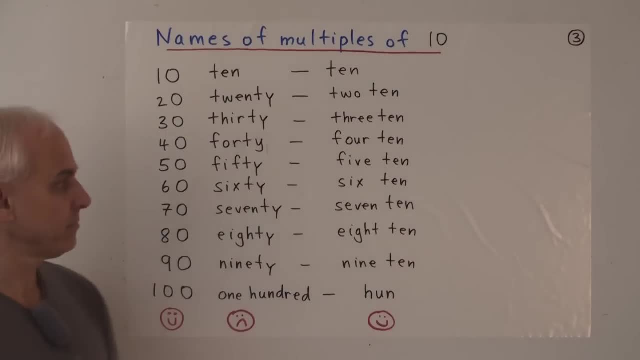 And then this one. we've already talked about 100.. Now, these names are a little bit arbitrary, but they're also obviously connected to the numbers 1, 2, 3, 4, 5, 6, 7, 8, 9.. 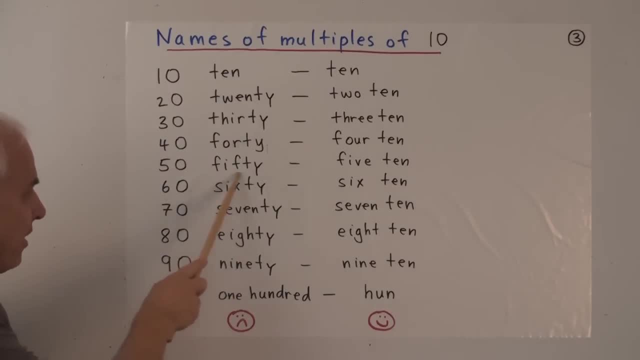 You can see the 9 there. You can see an 8 there, A 7 there, A 6 there, Kind of a 5 there, Something like a 4 there. The 3 there is a little bit more dubious. 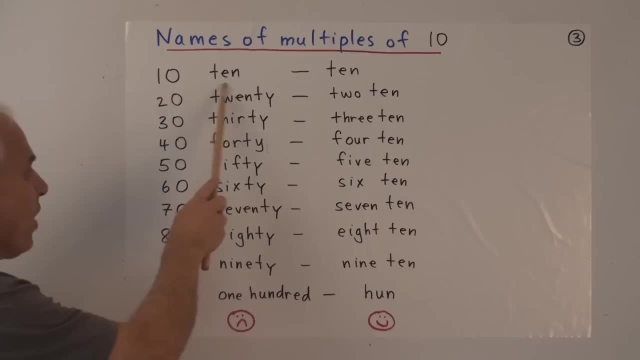 The 2, well, there's a bit of a 2 there And that's just one 10 by itself. So these names are a little bit arbitrary And we run into the same kinds of comments that we made about the numbers from 11 to 19.. 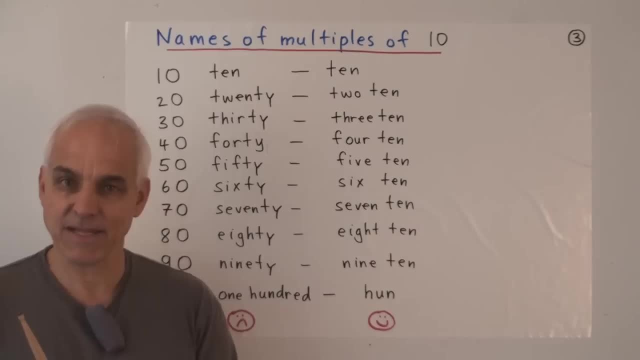 The fact that these numbers don't have really logical names, that there's not an obvious pattern to this, means that students have to memorize these numbers And that adds an extra layer of difficulty in learning arithmetic. In fact, I'll confess to you that when I was writing these things down reasonably quickly, 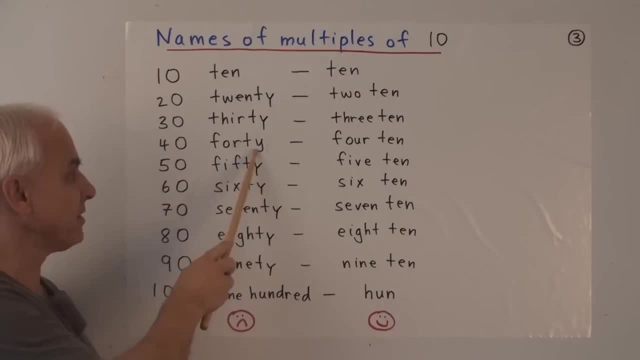 when I got to 40, I wrote F-O-U-R-T-Y Until I looked at it and said, no, that doesn't look right. So if you don't do this a lot, it's easy to get confused. Is there a 4 there, like F-O-U-R, or is it 40?? 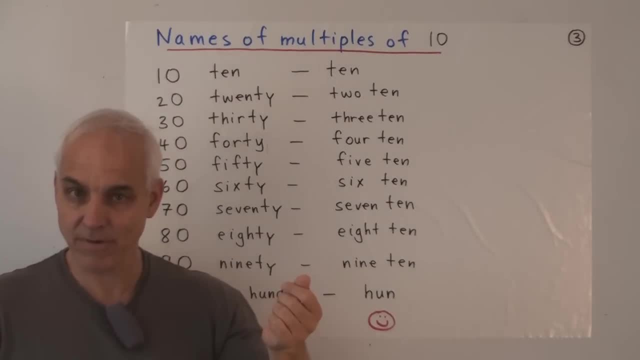 Remember 14,, which was a similar question, Which was a similar kind of number: 14,, 40, much the same. The 14 does have an F-O-U-R there, While the 40 doesn't. So you have to remember idiosyncrasies like that. 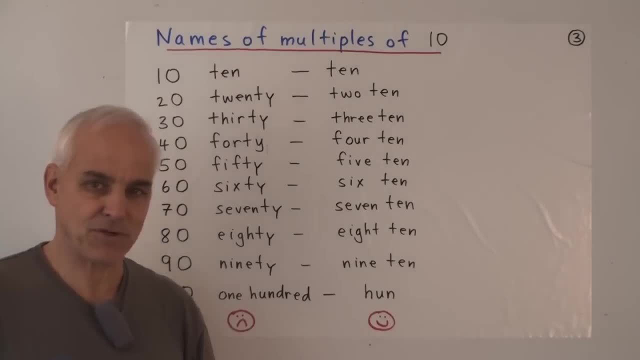 And for a lot of us, remembering things for which there's no good reason is a little bit hard. Okay, so I did propose some alternate kind of naming system for the numbers 11 to 19.. Let me go ahead and continue with that. 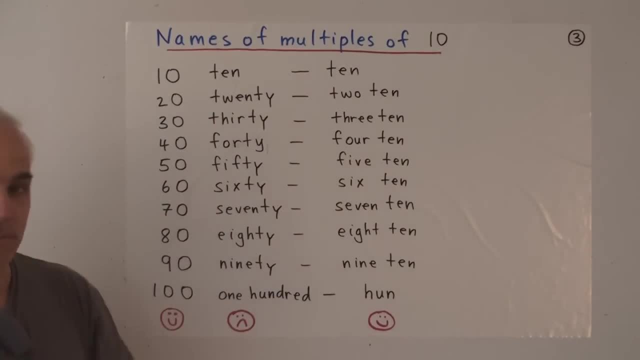 I'm going to take this idea, that vein, and give some alternate possible names for these numbers. Obvious kind of names are 10, as before, And then 210, 310, 410, 510, 610, 710, 810, 910. 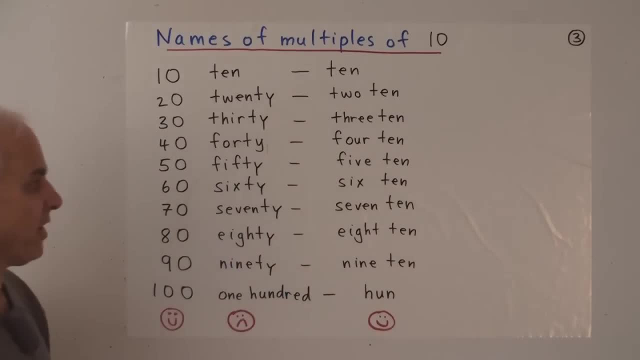 That makes it completely obvious, completely clear, what the pattern is and there's nothing really extra that needs to be memorized. And I think there are certain languages in which this kind of system is used And, pretty clearly, students using this kind of nomenclature. 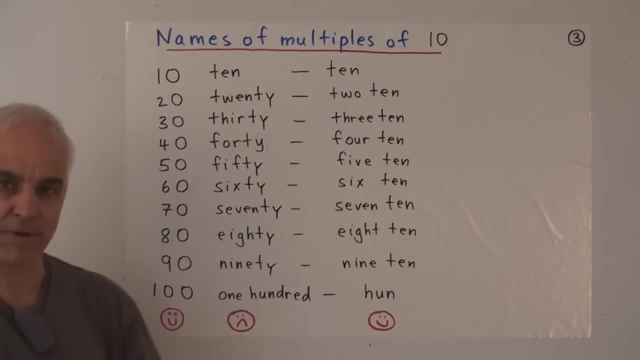 have an advantage over students who are forced to use something like this. I might say that English is not the worst language in this regard. French, which is a very beautiful language, of course, does have even more idiosyncrasies when it comes to naming these kinds of numbers. 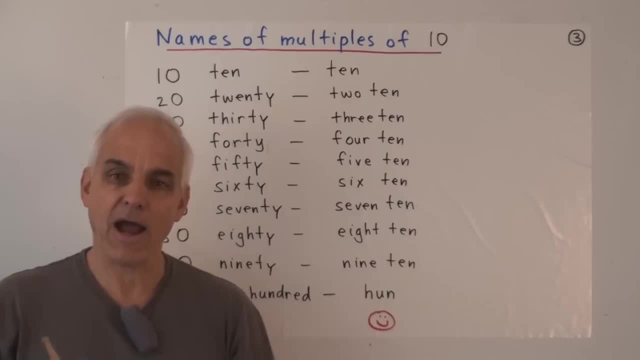 And I'm not sure about other languages- probably there's quite a variety of logical consistency between various languages. It might be interesting to make a study of that And see, for example, how it correlates to students' acceptance of early arithmetic. Alright, so we'll of course stick with this primarily. 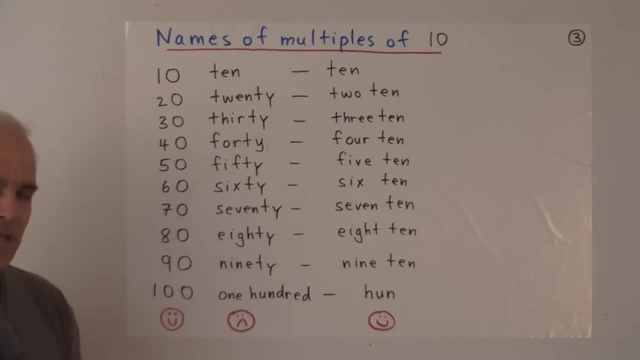 but every so often I might throw one of these things in just for fun. So just keep in mind that we have a kind of an alternate possible notation for these, But if you're a student, you're going to have to learn these names for the multiples of 10.. 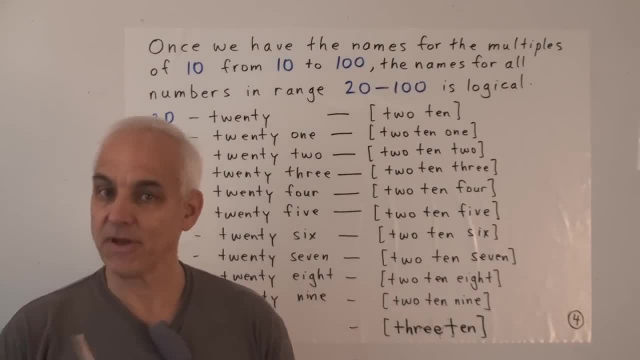 Very, very important. Once we have the names for the multiples of 10, from 10 to 100,, then the remaining numbers, from 20 to 100, have very logical, consistent names. We just add 1,, 2,, 3,, 4,, 5,, 6,, 7,, 8,, 9. 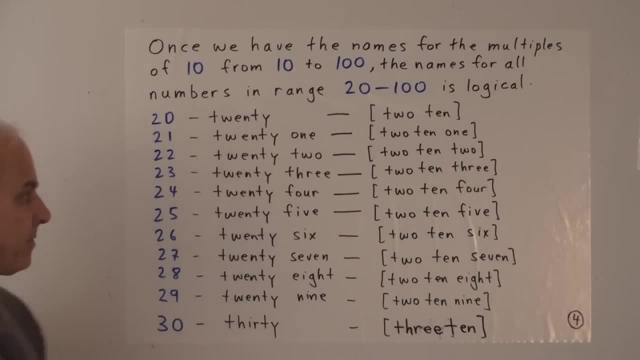 to the corresponding multiple of 10. So, for example, from 20 to 30, the numbers are 20, then 21,, 22,, 23,, 24,, 25,, 26,, 27,, 28,, 29, and 30.. 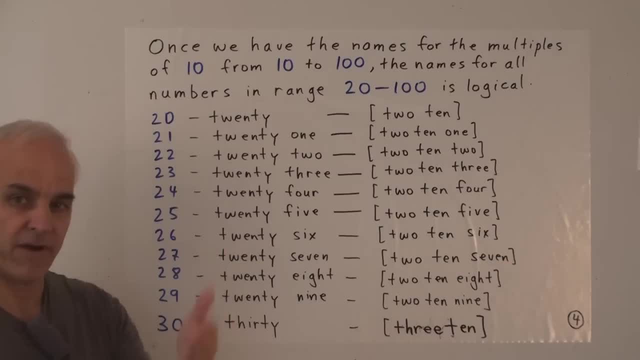 And the pattern continues that way for all the various multiples of 10.. So from 30 to 40,- it's the same kind of thing- 30, and then 31,, 32,, 33, and so on down to 40.. 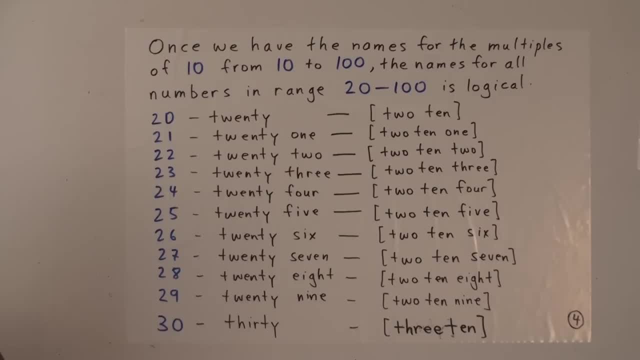 In this simplified, more logical presentation that I'm half suggesting, the corresponding names would be something like this: 25 would be written 2, 10, 5.. 2, 10, representing that digit there. 5, representing that digit there. 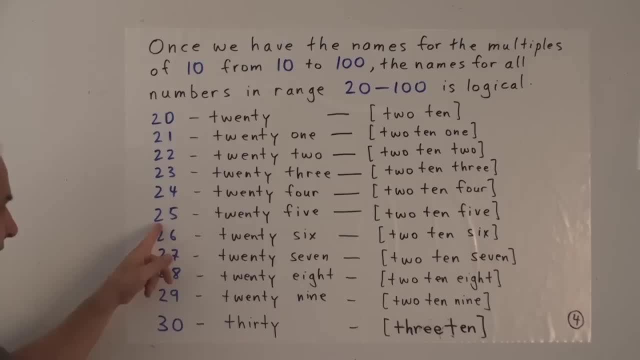 We're just reading left to right, taking into consideration: this is the 10s and that's the 1s. So the logic there is quite simple: Quite, consistent and similarly with this one. So we have the numbers from 1 to 100 now. 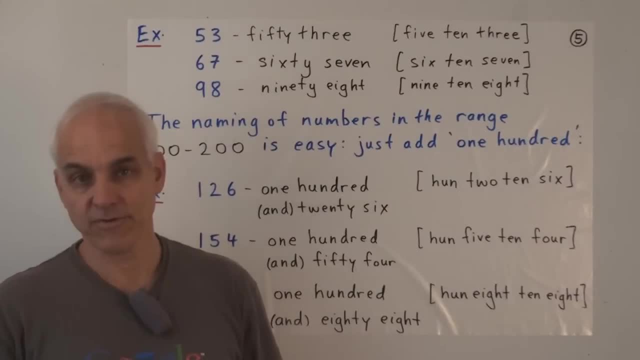 and we've given names to all of them. So a few examples. This number is 53, because it consists of 50, which is the multiple of 10, plus 3.. 5 10s, 3 1s makes 53.. 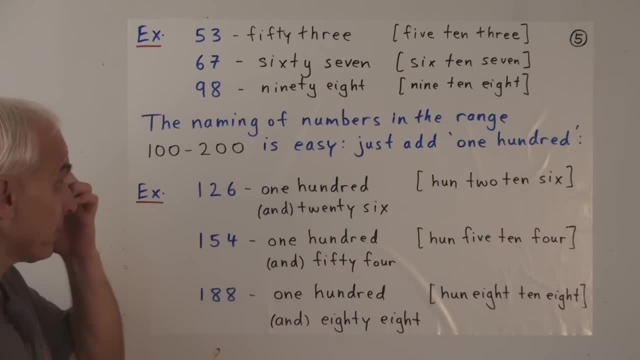 In our simplified formulation that would be 5, 10, 3.. This one 67, or 6,, 10, 7, and 98, or 9,, 10,, 8.. So once we have the numbers from 1 to 100 down. 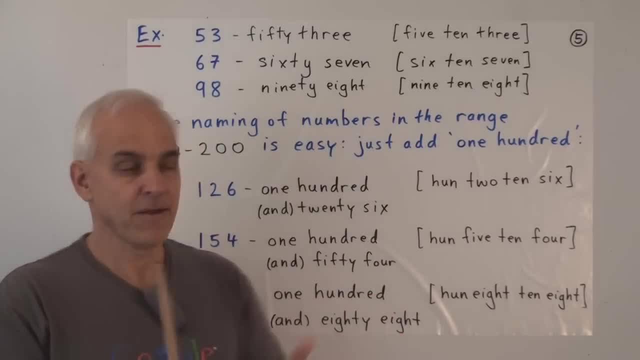 then the numbers from 100 to 200, say, are pretty straightforward. All we have to do is just add 100 to the front. So this number here, which is 6, 1s, 2, 10s, 1, 100,. 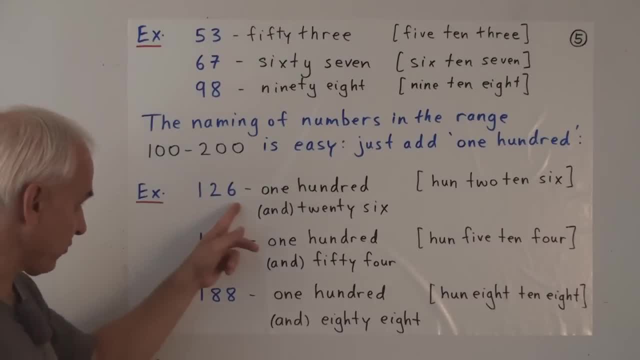 that's spoken how We read from left to right. So we read 100 and 26.. This too represents 2, 10s. so that's a multiple of 10, the multiple we called 20.. So 126.. 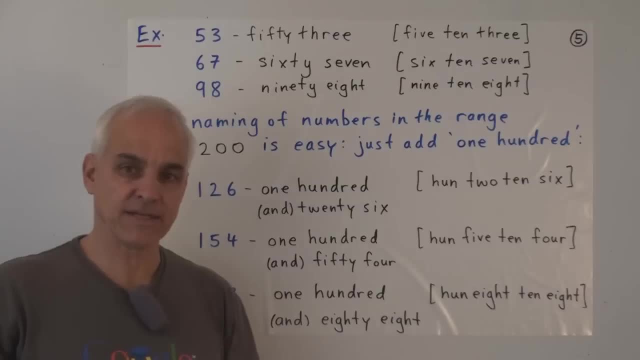 This word and is sometimes used and sometimes not used or used just a little bit. 126, people often say with just an n sound to represent that and I would suggest, in a simplified kind of formulation to think about 100. 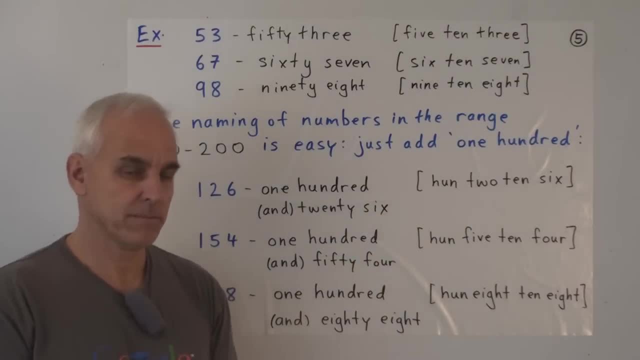 as being represented by the word hun. Maybe a little bit short, but short is good. So just like 10,. hun is the same kind of construction, So this would be hun 2, 10,, 6.. Might take some getting used to. 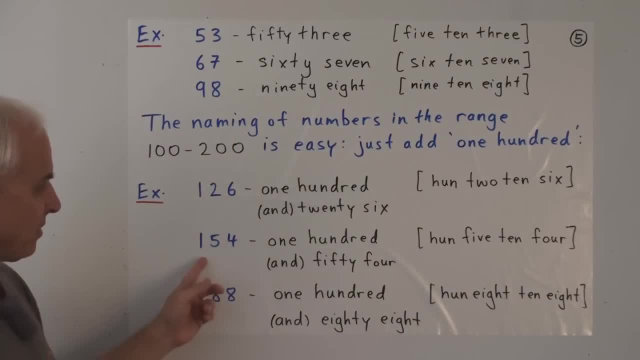 but this kind of thing is easier to say, certainly shorter than 154.. Hun 5- 10, 4.. 188, 188, or hun 8- 10, 8.. I'll just give some thought to this. 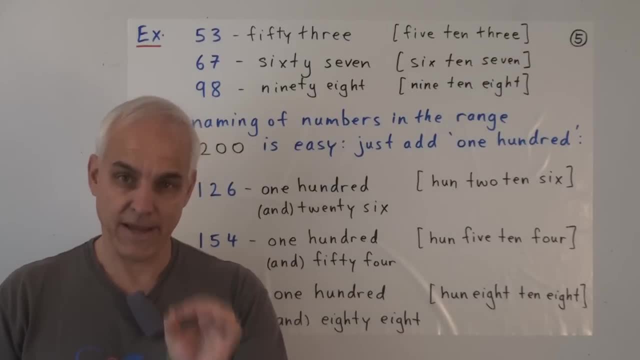 It's nice to have short words for important names, especially important names of numbers, ones that you use a lot. If you were counting from 100 to 200,, 101,, 102,, 103,, 104,, 105, and so on, 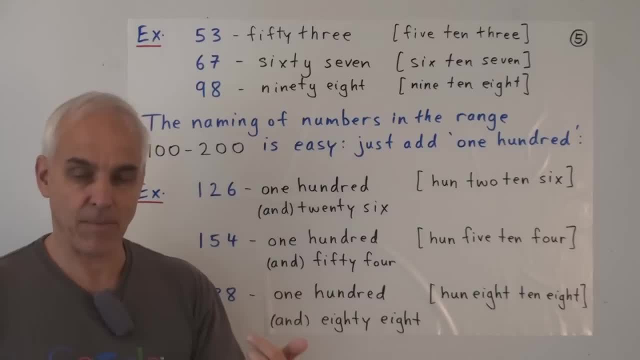 that 100 that you have to say all the time becomes a nuisance because it's long and also because we are obliged to say 1, and the 1 is really rather unnecessary. So we're now in control of the numbers, from basically 1 up to say 200.. 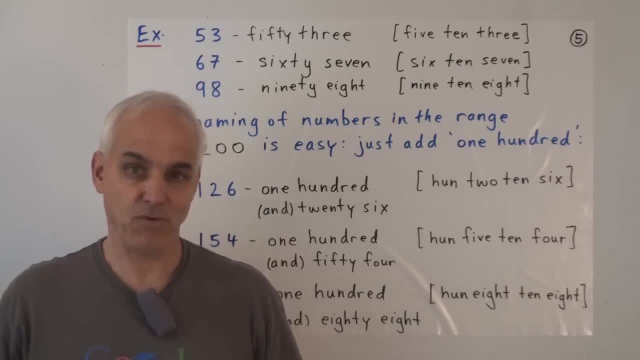 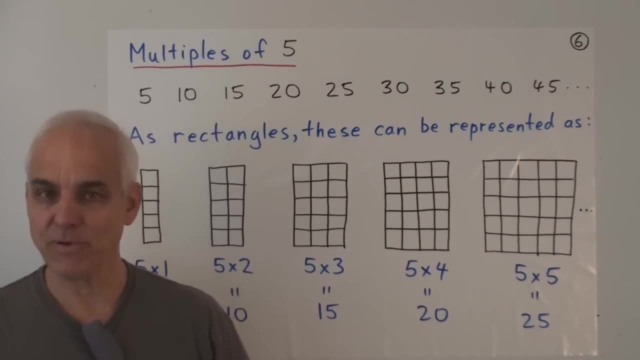 And now we can have a look at multiples of some other numbers. Now that we have good names for numbers, we can start talking about them a little bit more fluidly. So here are the multiples of 5.. What you get when you start with 5,. 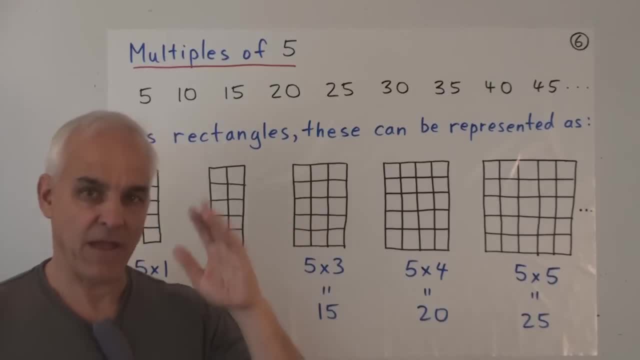 and then you add another 5,, and then you add 5,, and then you add 5, and you keep on adding 5.. That's what we mean by multiples of 5.. So 5, add 5,, you get 10.. 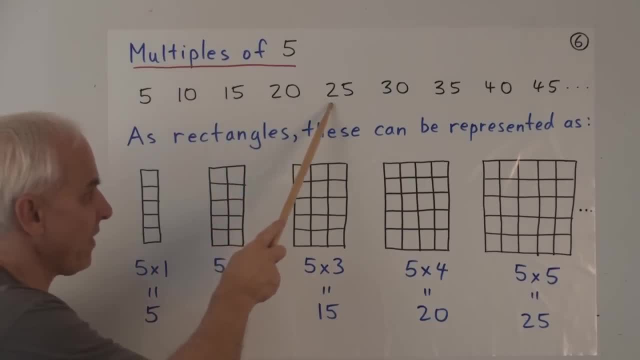 Add 5,, you get 15. And then 20,, and then 25,, and then 30,, and then 35,, and then 40,, and then 45. And we can represent those numbers also geometrically, in terms of rectangles. 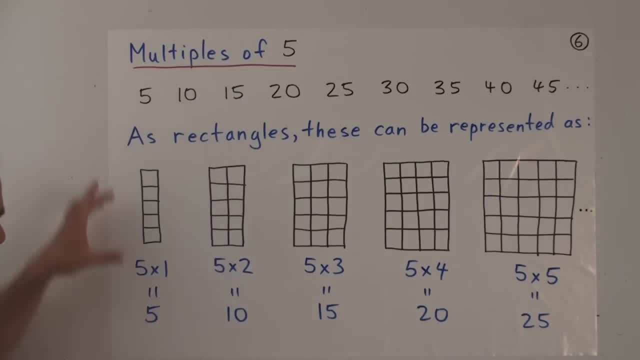 And that's a very nice thing to do. We're going to use rectangles which have 5 rows, So 5 times 1, there's that first rectangle. It has 1,, 2,, 3,, 4, 5 squares in it. 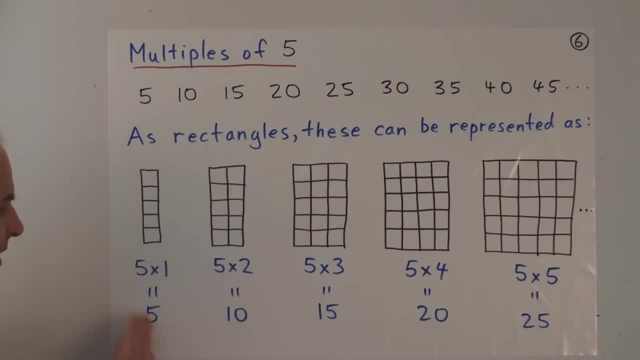 So it's another representation of 5.. 5 times 2, that's that shape rectangle that has 10 in it. That's a way of thinking about 10.. This way we can get more multiples of 5, just by extending the rectangles. 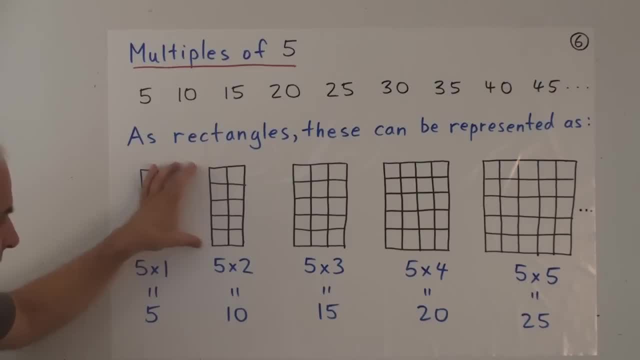 in this horizontal direction, always with the same height. So all of these rectangles- these are all multiples of 5, have the same height. They're all 5 rows high, 5 times 1,, 5 by 2,. 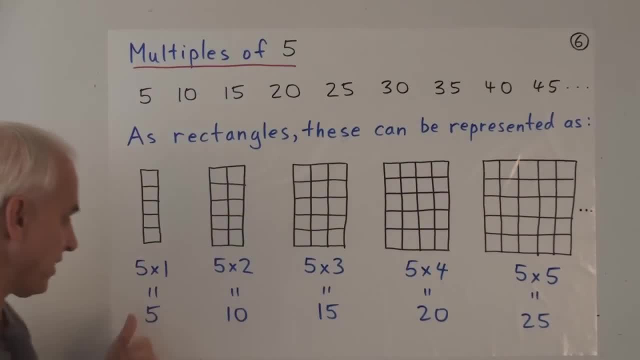 5 by 3,, 5 by 4,, 5 by 5, these are the numbers 5, 10,, 15,, 20, and 25.. And, of course, we can keep going. So it's very important for the students. 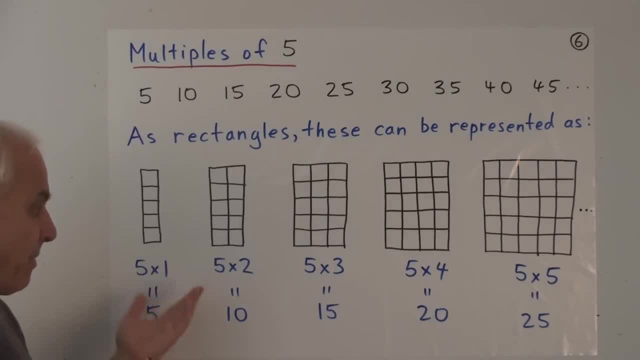 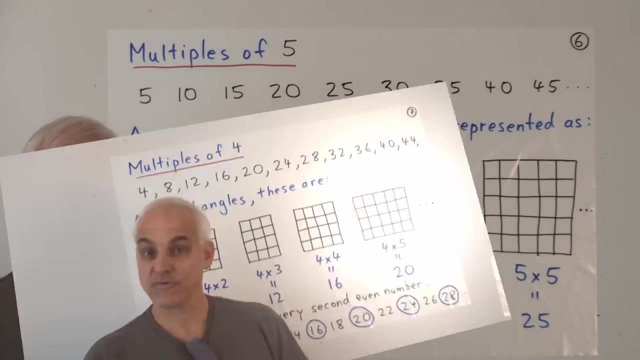 to think in terms of multiples of a number like 5, in terms of rectangles. This two-dimensional aspect of numbers, which are products, goes back to the ancient Greeks and has a lot to recommend it. After getting down multiples of 5, the next simplest system of multiples: 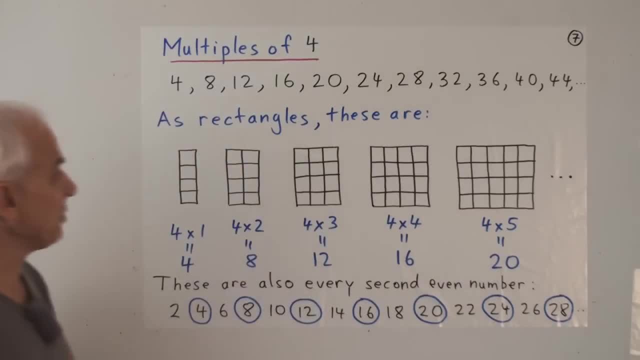 are the multiples of 4.. The multiples of 4 are 4, then 4 plus 4 is 8,. 8 plus 4 is 12,. 12 plus 4 is 16,. keep on adding 4,, 20,. 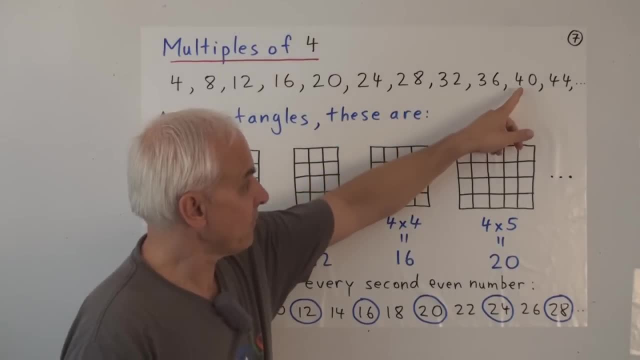 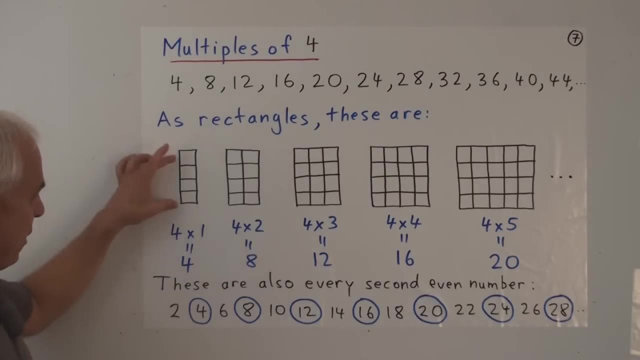 24,, 28,, 32,, 36,, 40,, 44, and so on. These also have representations as rectangles. Now there are 4 squares high: 4 by 1,, 4 by 2,, 4 by 3,. 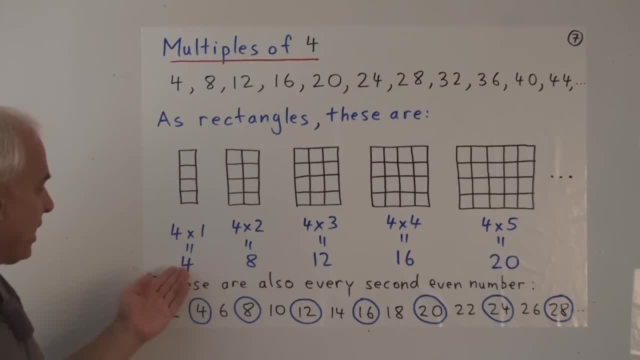 4 by 4,, 4 by 5.. These are also ways of representing the numbers 5,, 4,, 8,, 12,, 16, and 20 when we're thinking of them as multiples of 4.. So here's that number 20,. 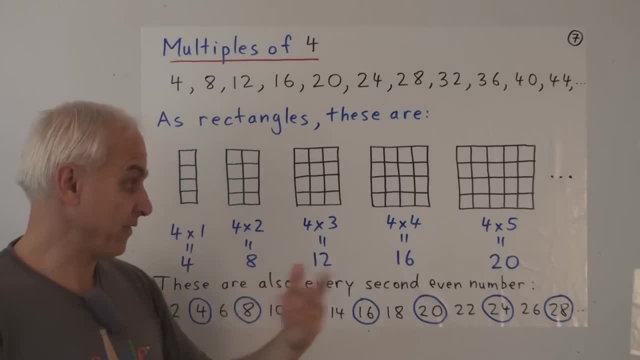 which we also had another way of thinking about that. We thought of that as a multiple of 5 as well. So this is a multiple of 4, it's a multiple of 5, it's also a multiple of 2, because it's an even number. 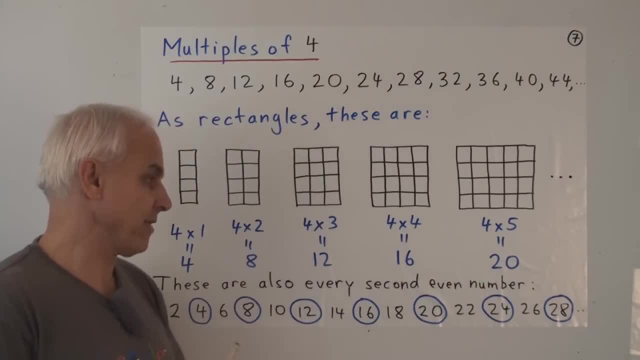 and it's also a multiple of 10.. So that's not a problem. Numbers can be multiples of lots of other numbers, And so a number like 20 can have different representations in terms of a rectangle. This is one of them. We can also represent it as a. 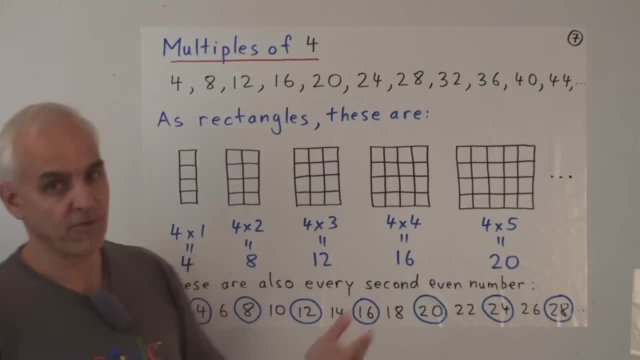 rectangle with 2 rows and 10 columns, or 5 rows and 4 columns. So the multiples of 4 are reasonably easy because we've sort of seen them before. They're really every second one in the sequence of even numbers. So here are all the even numbers. 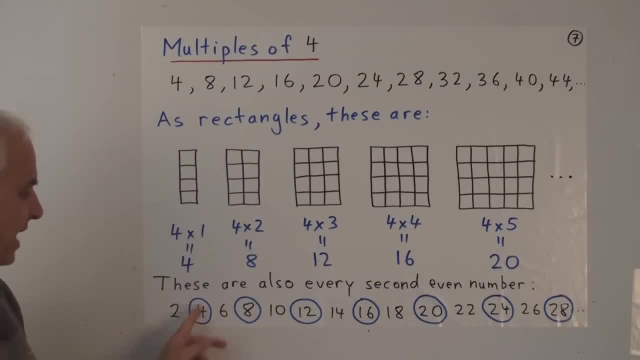 And the multiples of 4 are just every second even number: 4, then 8, then 12, then 16, then 20, then 24, then 28.. That makes sense because with the even numbers we're going up by 2 each time. 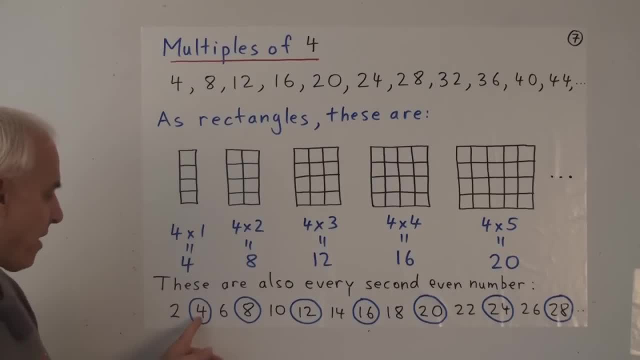 and with the multiples of 4 we're going up by 4 each time, So it's sort of like 2 plus 2,, 2 plus 2,, 2 plus 2, and so on. Multiples of 4.. 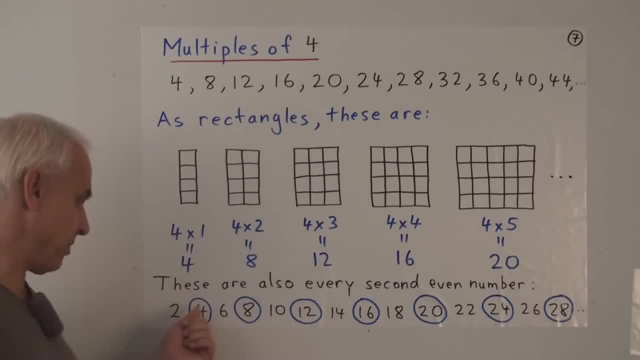 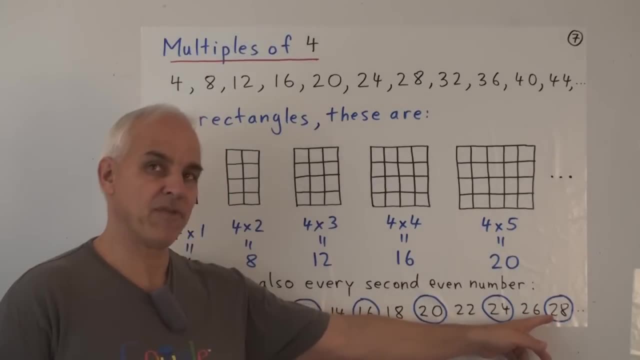 So students should work their way through these. They should be able to generate these multiples in their head by doing little additions. Then, for the next one, what's 28 plus 4?? They have to figure it out. It's 32.. 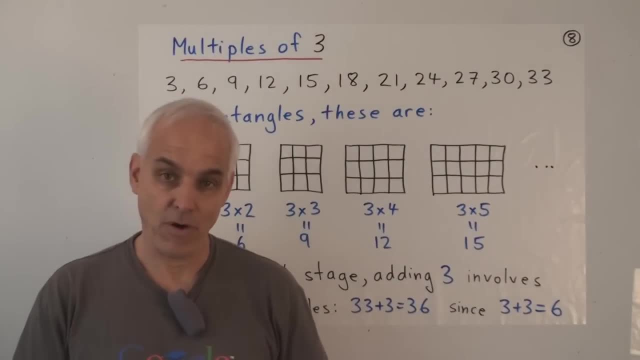 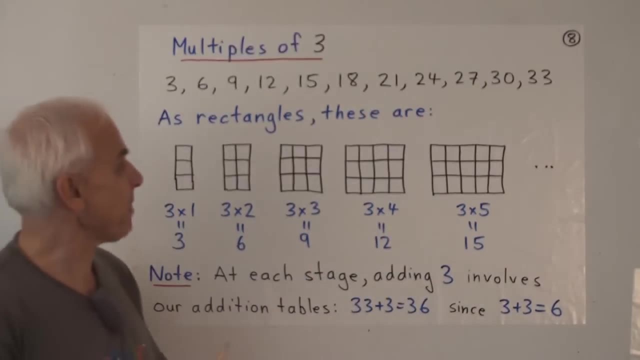 And so on. And then, after multiples of 4,, the next natural multiple system is that of multiples of 3.. Particularly pleasant pattern, I think: 3,, 6,, 9,, 12,, 15,, 18,, 21,. 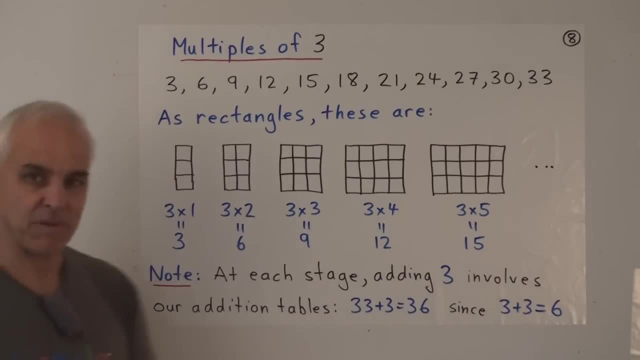 24,, 27,, 30,, 33, and so on. Biggest 3,, after all, is many people's sort of favorite number. It's a very nice number to work with, Pretty small. You can easily see what's going on. 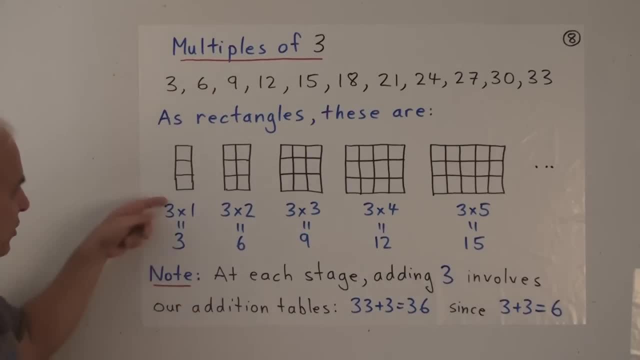 It's a little bit more interesting than 2.. There's 3 by 1,, which is 3,, 3 by 2,, which is 6,, 3 by 3,, which is 9,, 3 by 4,. 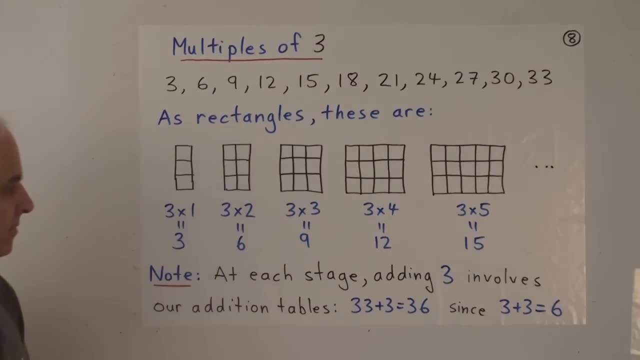 which is 12,, 3 by 5,, which is 15, and so on. So at each stage we get the next one by adding 3.. So, for example, the next one after 33, we would get by adding 3.. 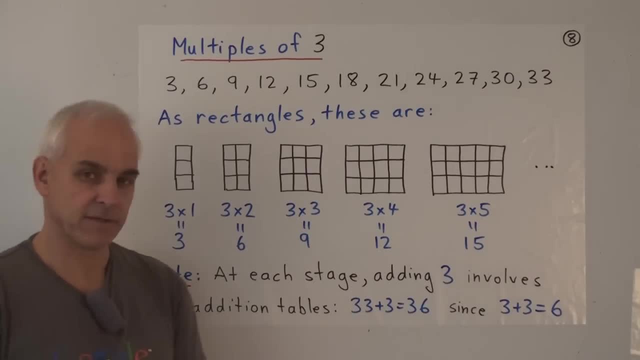 33 plus 3 equals 36.. And how do we know that? Well, you can either sort of do it in your head: You have 33, and then you have to add 3, so 34,, 35,, 36.. 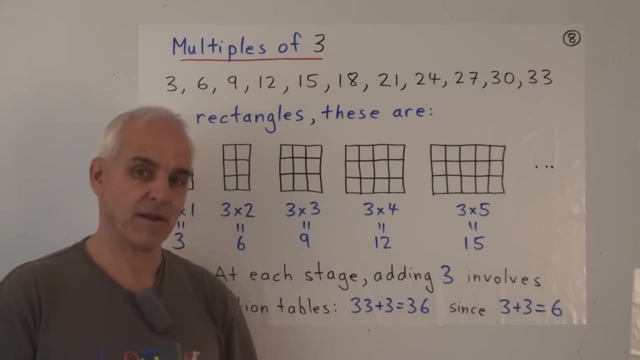 And many students will do that calculation that way. But another way for them to think about it is we're adding 3 to the 3 units that are here. So it's really a case of knowing the addition table of what is 3 plus 3.. 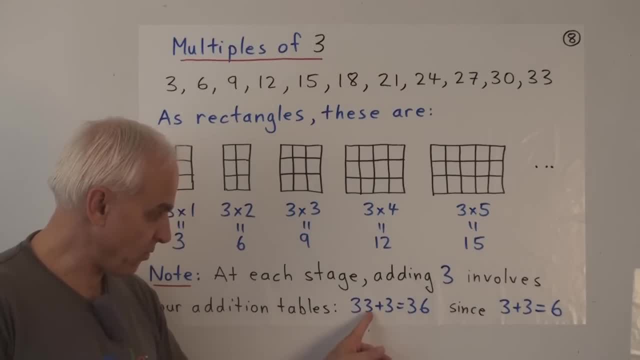 This is 3 ones. Here we have 3 tens and 3 ones, So we're adding these 3 ones to the 3 ones which are already here to get 6 ones. The number of tens in this case doesn't change. 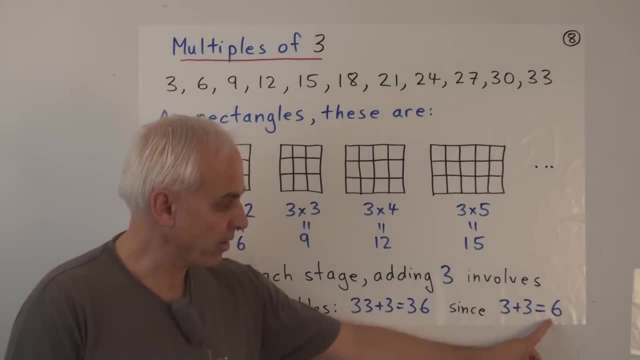 So ultimately, this is a consequence of this simpler rule that 3 plus 3 equals 6. And so if a student knows this automatically without having to use fingers, then they can do this automatically because 33 plus 3,. 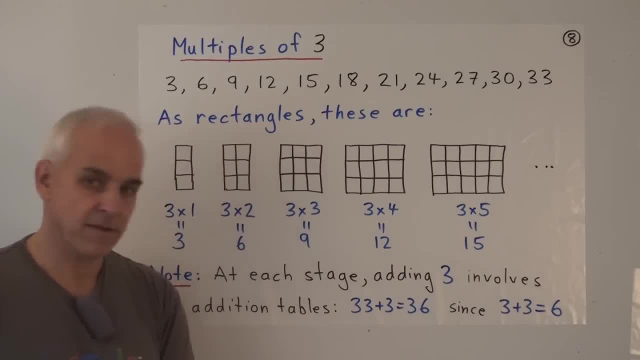 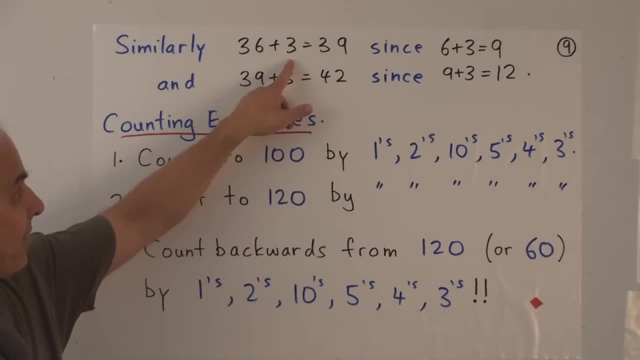 the two 3's here are the ones that add to get 6.. Similarly, when we get to 36 and we want to add 3, then it's the 6 and the 3 that are combining to give the 9.. 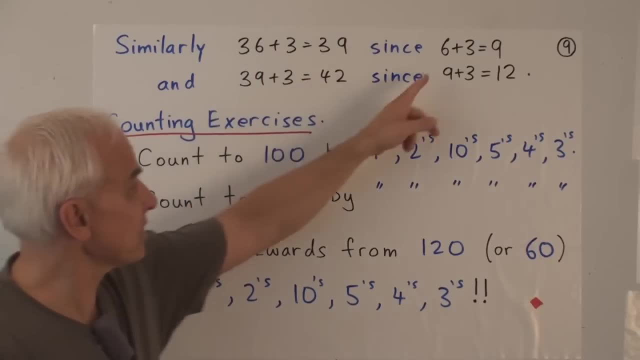 36 plus 3 is 39,, because 6 plus 3 is 9.. That's the essential knowledge that's required. Of course, you can do it by fingers: 36,, 37,, 38,, 39, there, we've just added 3.. 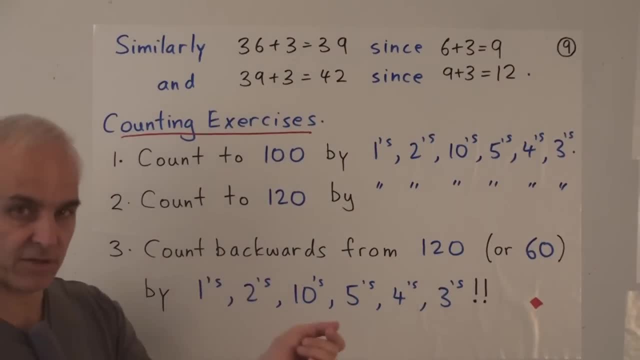 But it's probably better for the student eventually to realize that it's because 6 plus 3 equals 9, that 36 plus 3 is 39. This is 3 tens and 6 ones, and we're adding 3 ones. 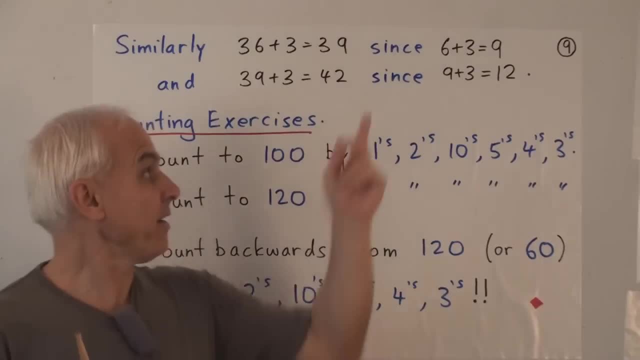 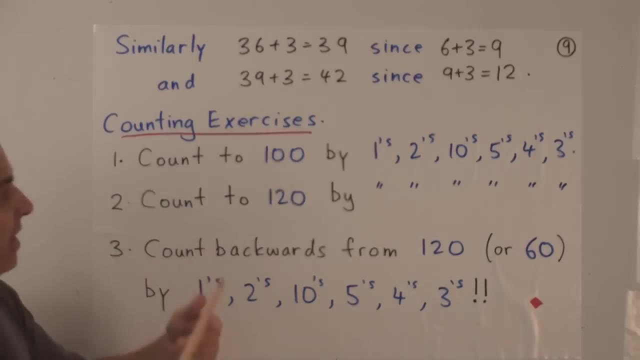 so the 6 ones and the 3 ones are adding to make 9 ones, and the 3 tens are sitting over there just as they were at the beginning. At the next step from 39, adding 3 more, we get something a little bit more involved. 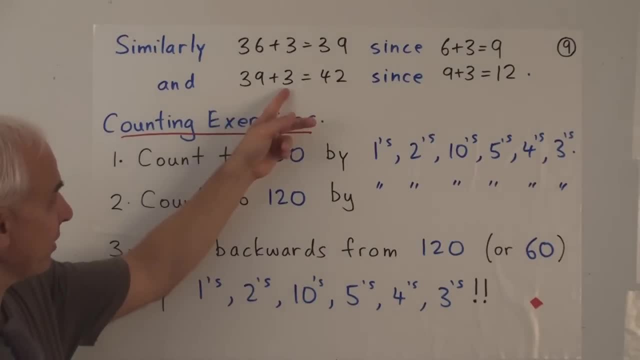 because we have to carry So 39 plus 3, well, with fingers 39,, 40,, 41,, 42, and the student should also realize that's because the 9 plus 3 is 12.. When we add 9 ones and 3 ones, 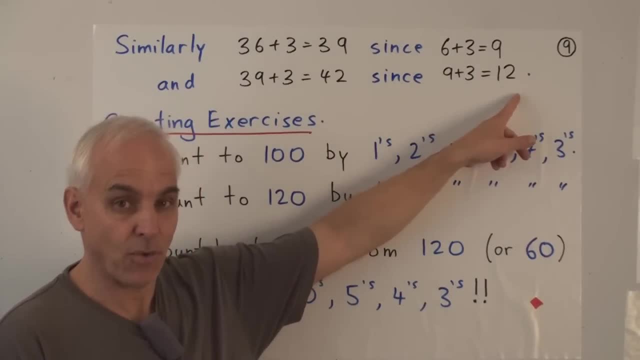 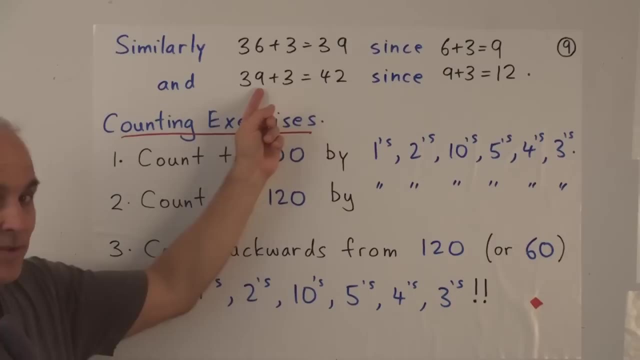 we get 12,, which is actually 10, 2.. It's 1 ten and 2 ones. So if we're starting with 39,, which is 3 tens and 9 ones, we add 3,, then the 9 ones here and the 3 ones here. 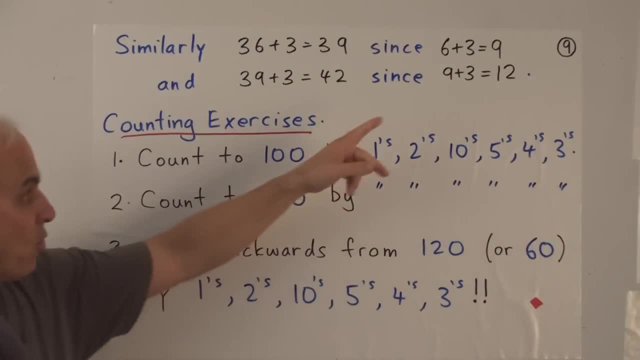 are combining to give us 10 and 2.. So one of those tens adds with the 3 tens we already have to give 4 tens, And this is admittedly simplified if you think of this as being 3, 10, 9.. 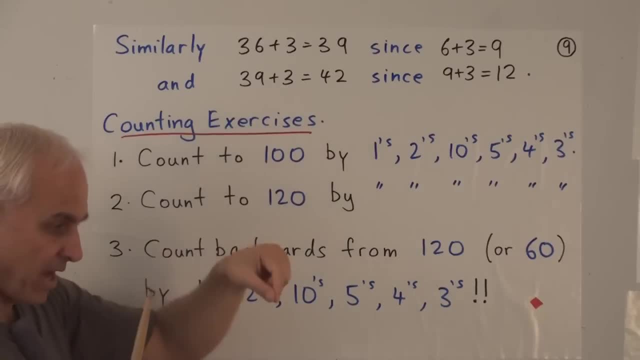 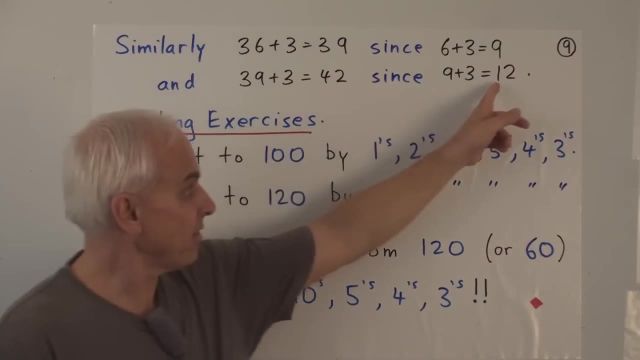 So that way, 3, 10, 9 plus 3, well, the 9 and 3 is giving 10, 2.. So 3, 10, 9 plus 3 equals 3, 10 plus 10, 2.. 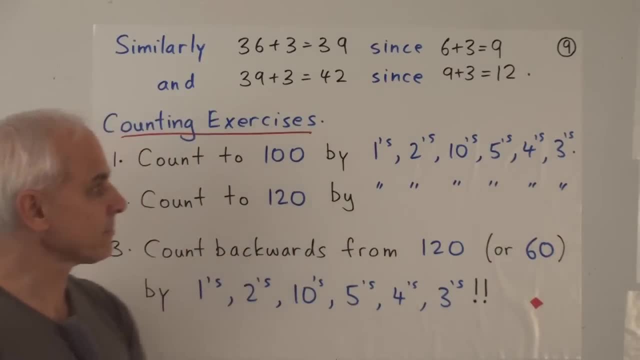 All together 4, 10, 2.. Alright, so there's lots of work to be done here. concrete work, working through calculating multiples, seeing how the carrying goes from one multiple of 10 to the next, Very explicit kind of work. 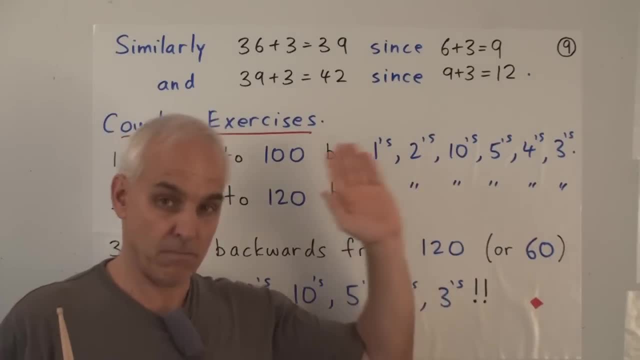 that has to be done. There's weeks of work, months of work for young students in mastering the contents of this particular lecture. The lecture is relatively short but the amount of material is very large for a young student or a beginner at mathematics. 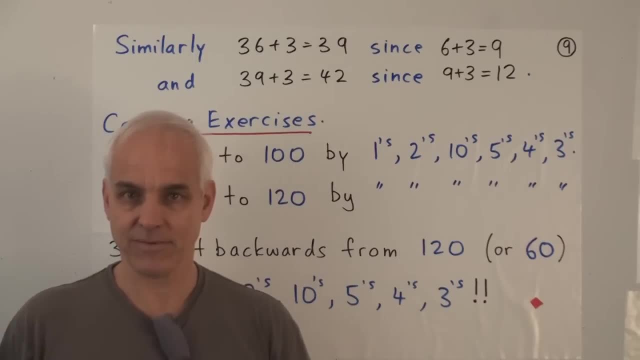 You want to become really familiar with these multiples, And there's perhaps no better way of becoming familiar with them than doing some exercises like this By counting with these multiples. First of all, counting by ones, That's the absolutely basic skill, Just counting up to some bigger number.